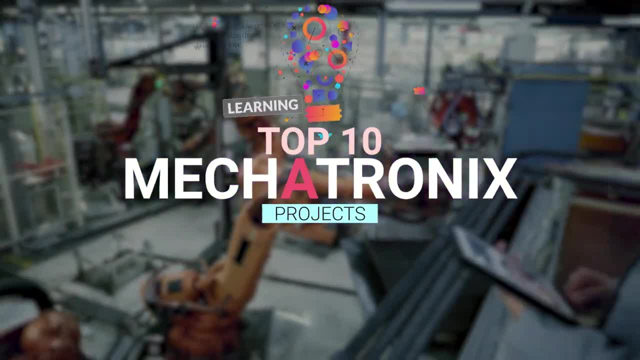 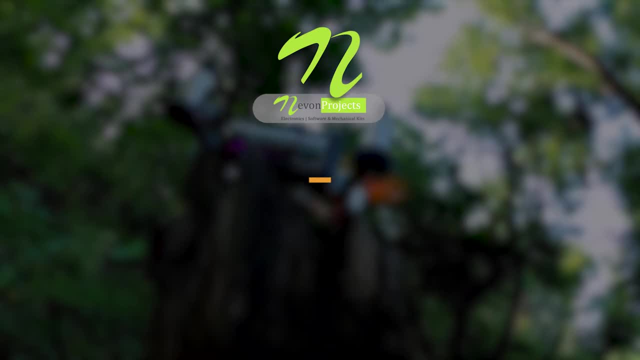 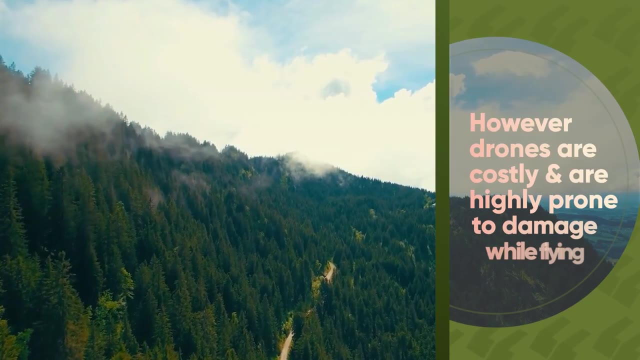 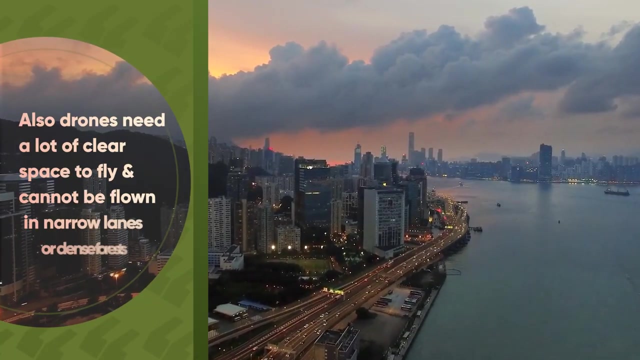 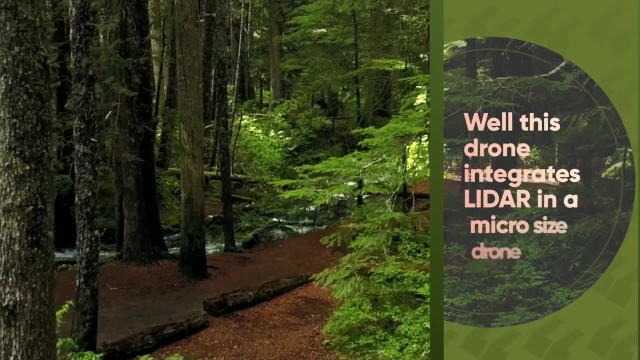 Today, drones are widely used for a variety of purposes. However, drones are costly and are highly prone to damage while flying. Also, drones need a lot of clear space to fly and cannot be flown in narrow lanes or dense forest. Well, this drone integrates LIDAR in a micro-sized 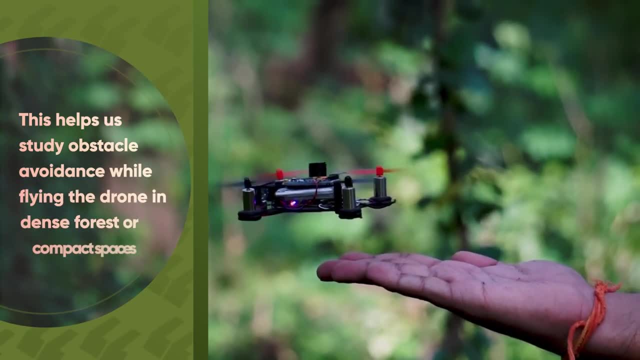 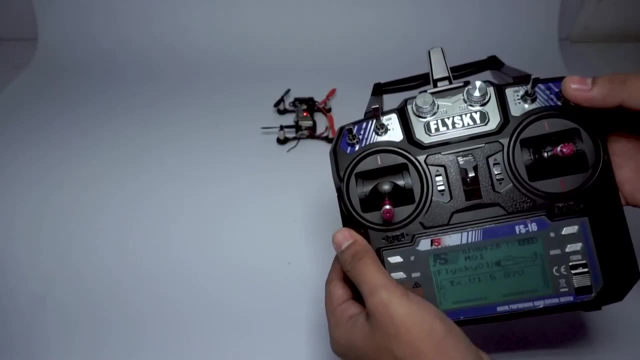 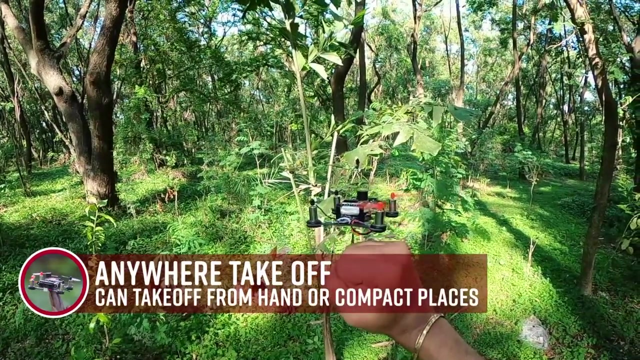 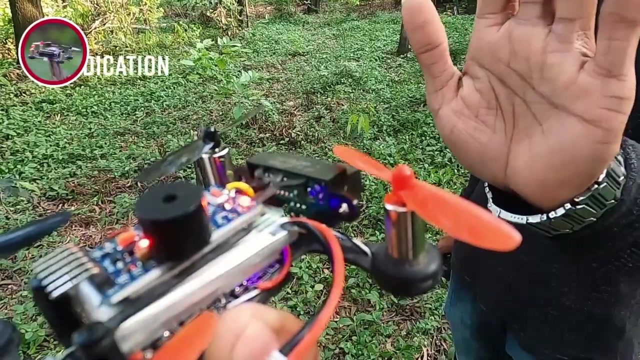 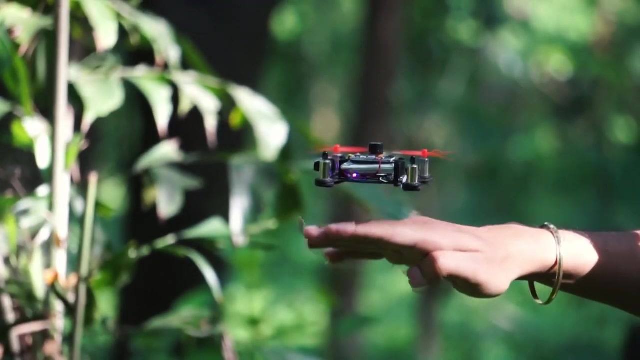 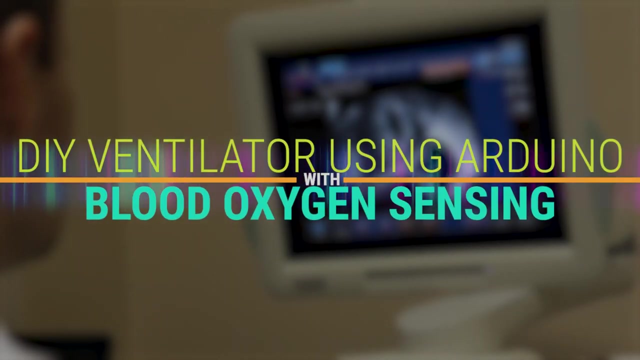 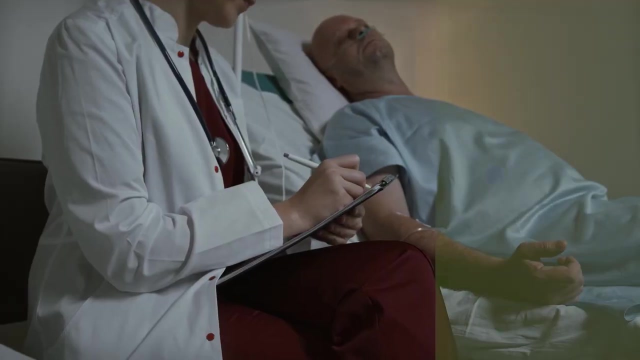 drone, and this helps us study obstacles: avoidance while flying the drone in dense forest or compact spaces. DIY Ventilator Using Arduino with Blood Oxygen Sensing Ventilators have been in the limelight in the COVID crisis. Developing low-cost ventilators is of key value in these times, so all those in need can afford one. 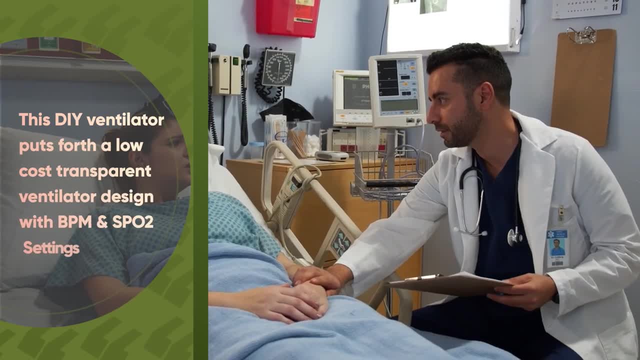 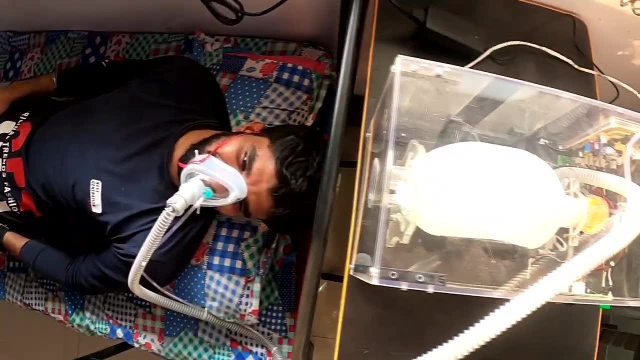 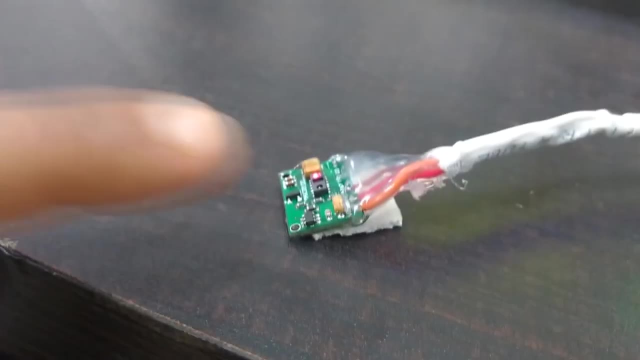 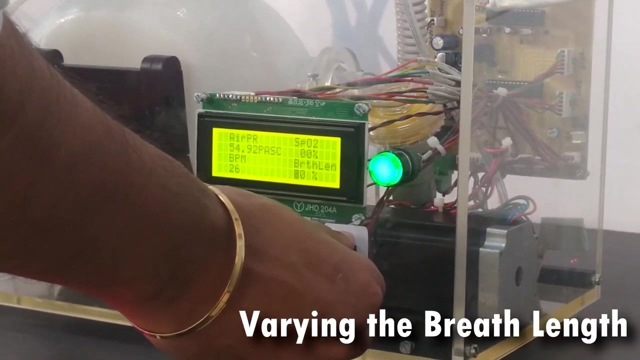 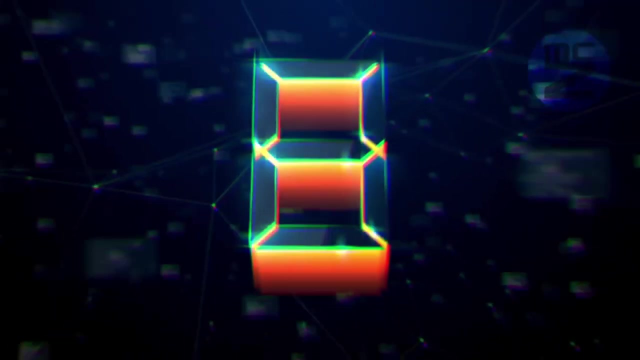 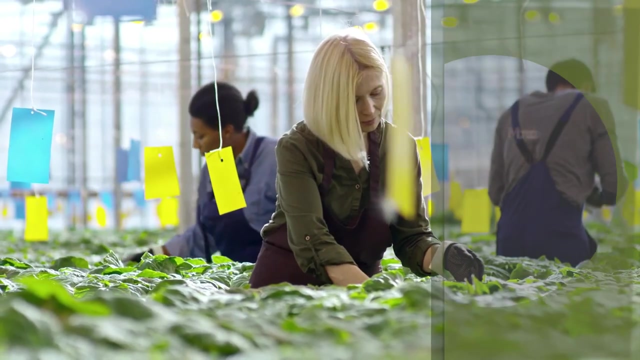 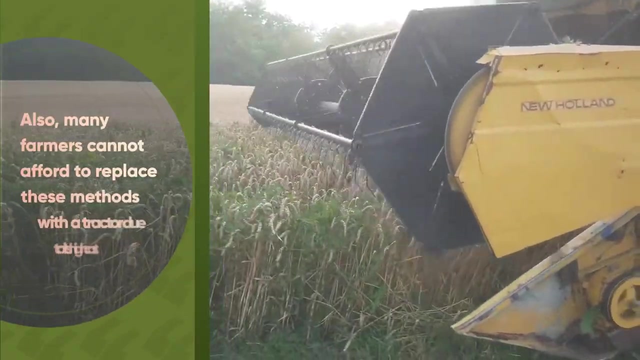 So this DIY Ventilator puts forth a low-cost, transparent ventilator designed with BPM and SPO2 settings. Portable Electric Power Tiler Machine Manual. farm tiling is one of the most labor-intensive operations in agriculture. Also, many farmers cannot afford to replace these methods with a tractor due to its high cost. 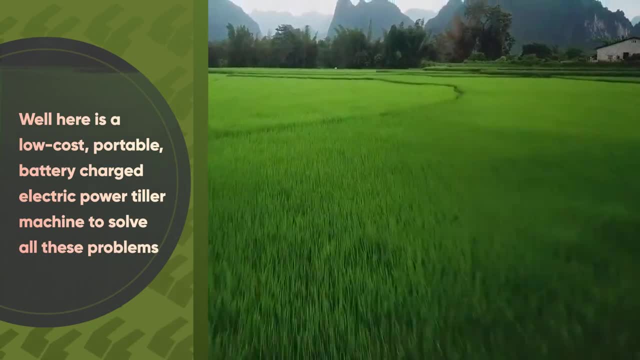 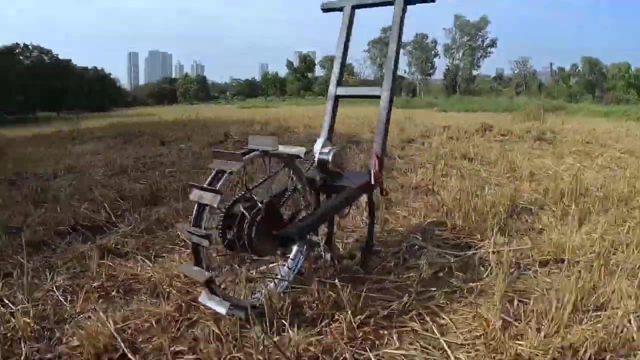 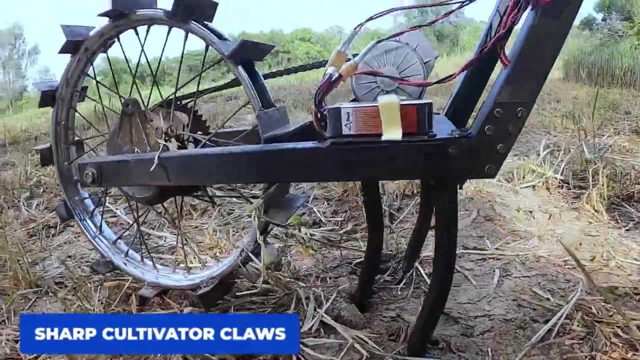 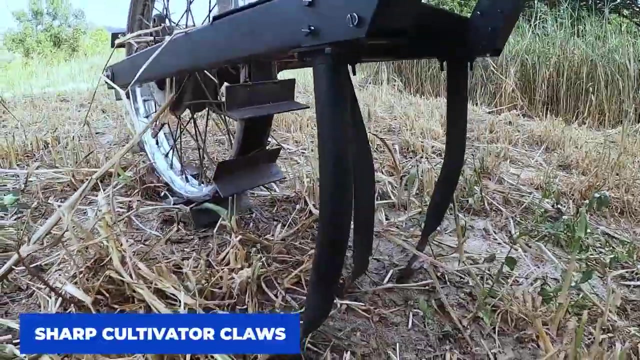 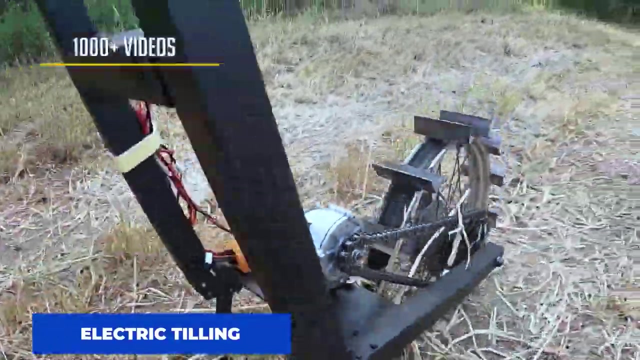 So here is a low-cost, portable, battery-charged electric power tiler machine to solve all these problems. In this video, we will be looking into a simple DIY breathing and aerodynamic design. So let's get started. DIY LIDAR Ventilator. 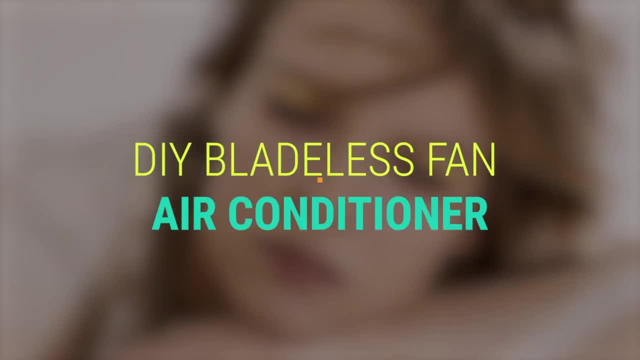 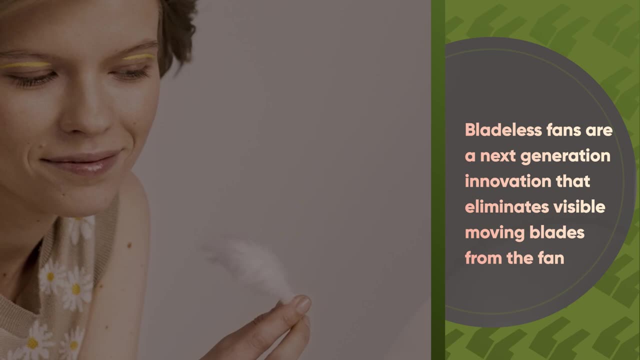 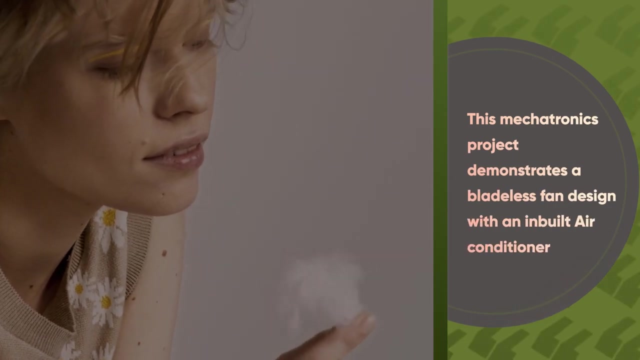 DL5 Speedometer, AC AeroTech- Air Conditioning- Thermometer Air Conditioning. DL5 Air Conditioning- Air Conditioning. Bladeless fans are a next-generation innovation that eliminates visible moving blades from the fan. So this mechatronics project demonstrates a bladeless fan design with an inbuilt air. 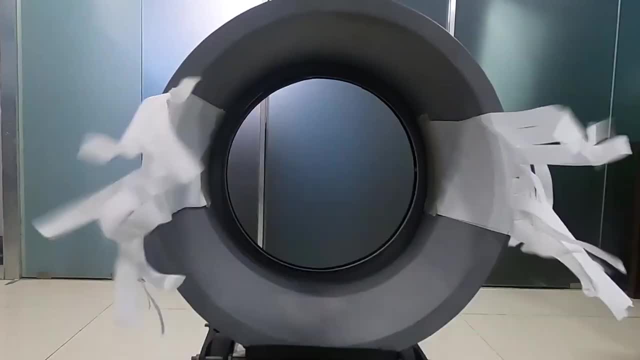 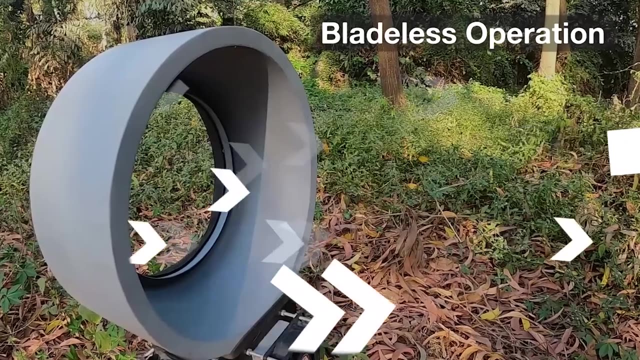 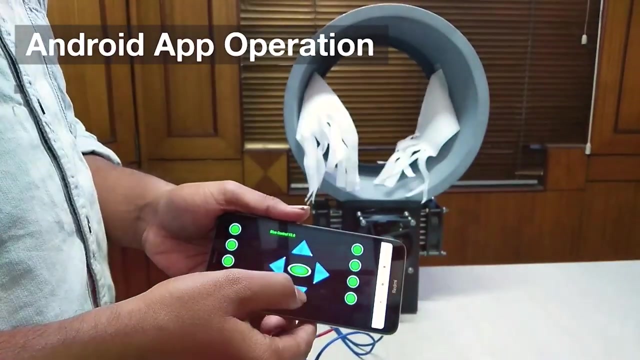 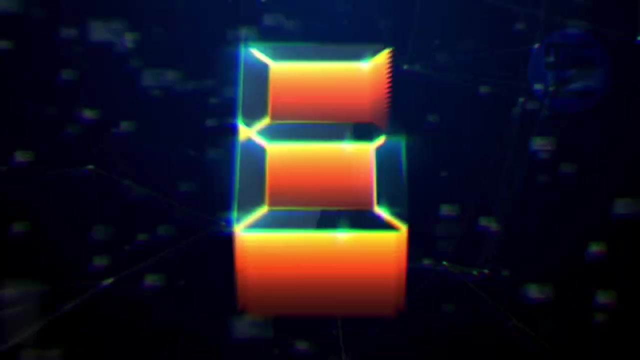 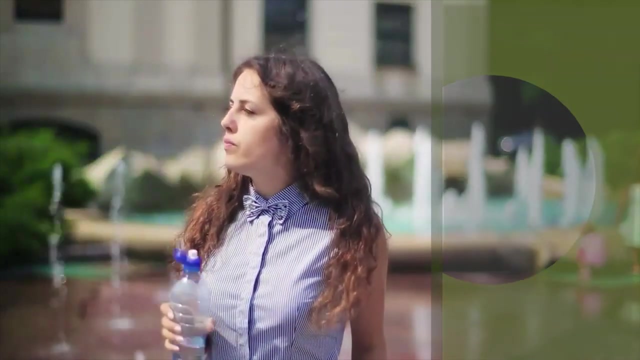 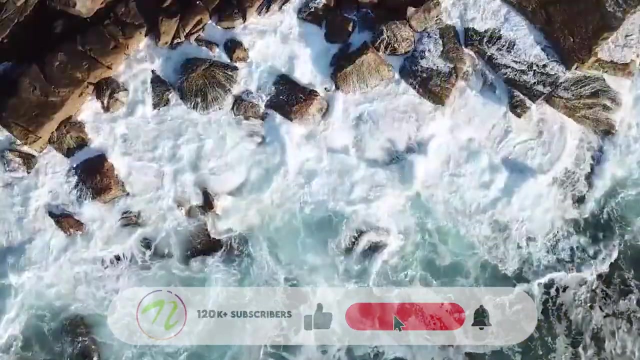 conditioner, Solar Seawater Desalination Machine. On an average, over 1.1 billion people over the globe lack proper access to fresh water. We all know 71% of Earth's surface is covered with water, But of that, only 3% is water. 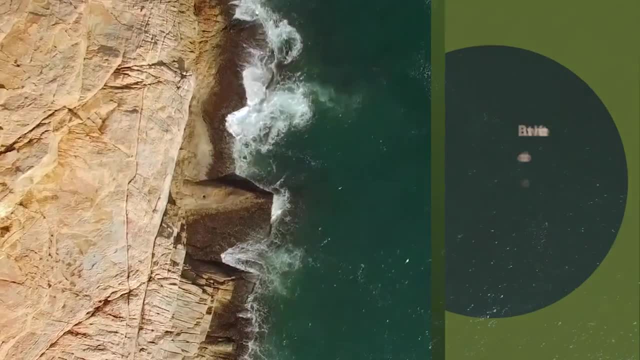 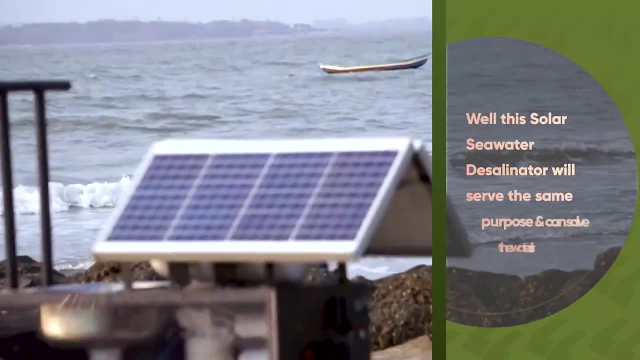 So how much can we actually do? Let's find out. water is drinkable, But what if we are able to convert the salty ocean water to fresh drinkable water? Well, this solar seawater desalinator will serve the same purpose, and 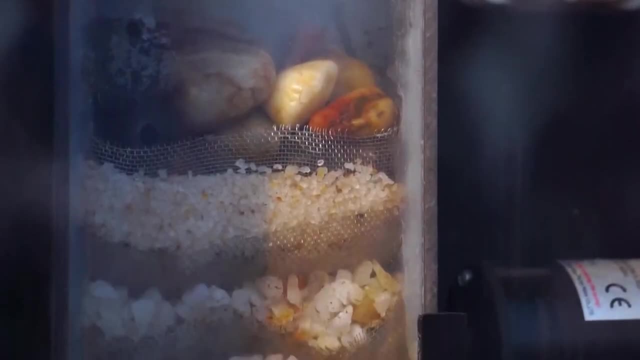 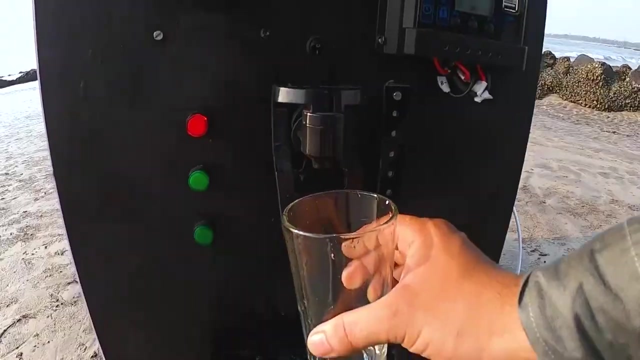 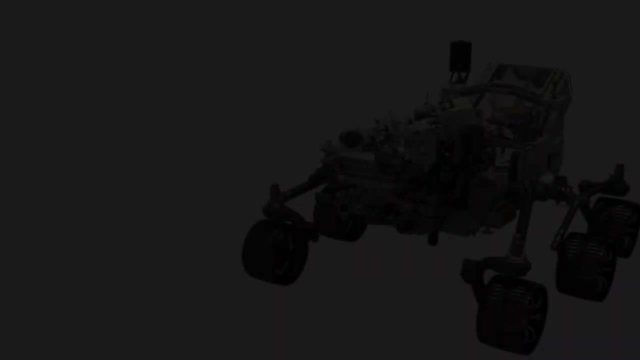 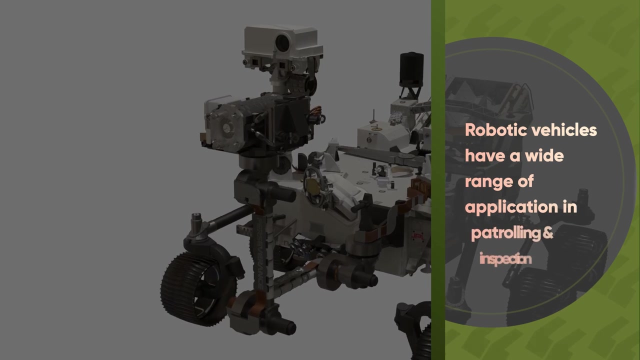 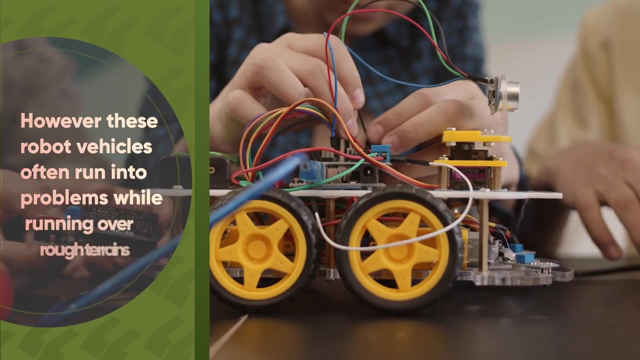 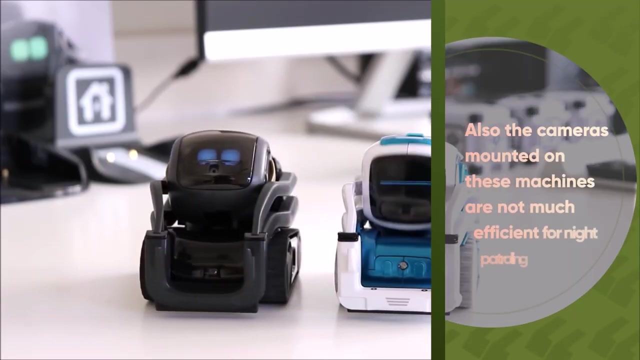 can solve the water crisis. Thermal vision RC robotic tank. Robotic vehicles have a wide range of application in patrolling and inspection. However, these robot vehicles often run into problems while running over rough terrains. Also, the cameras mounted on these machines are not efficient for night. 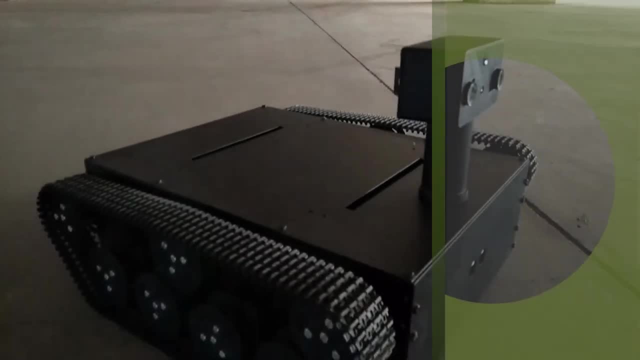 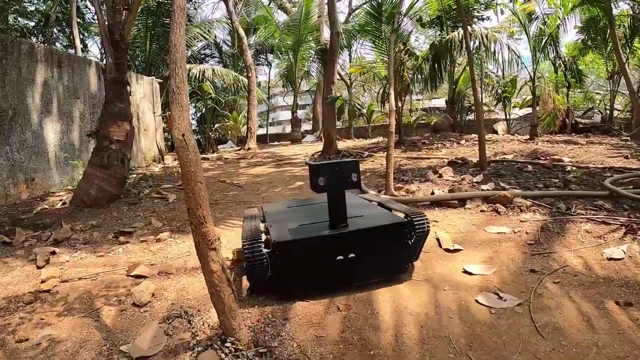 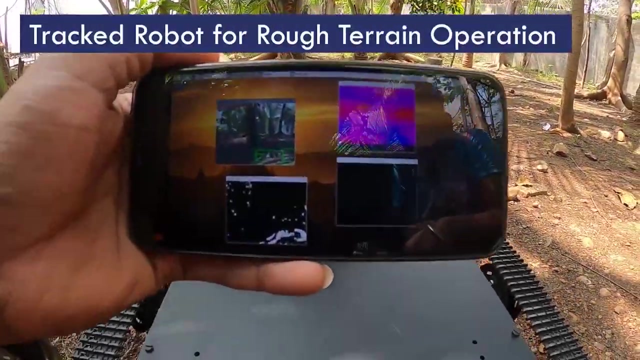 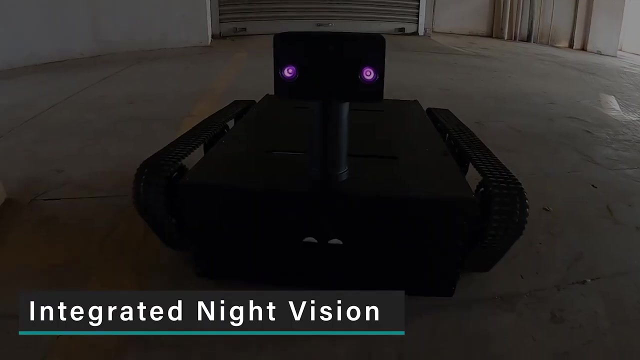 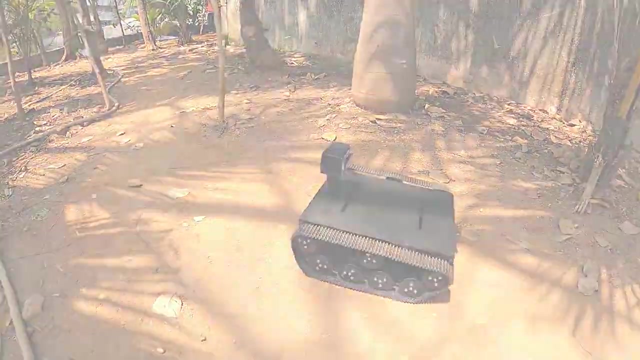 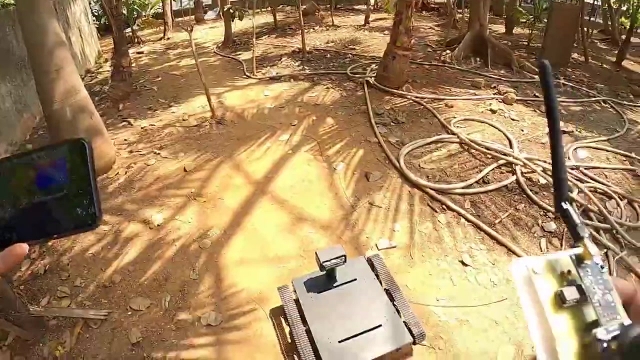 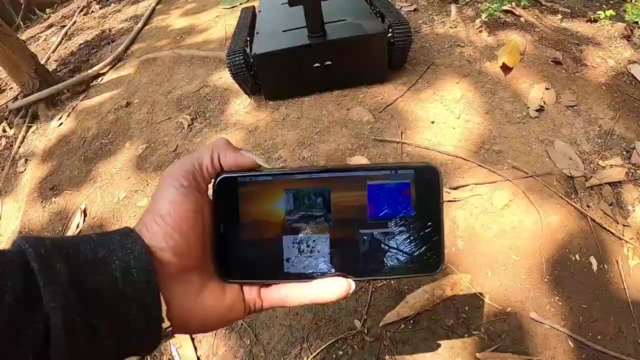 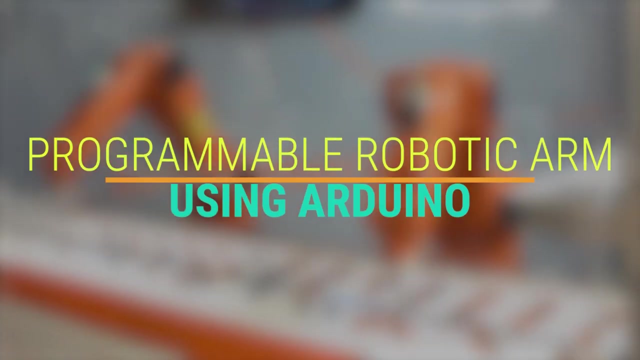 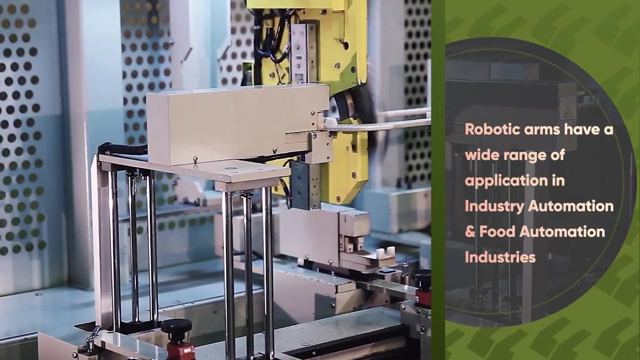 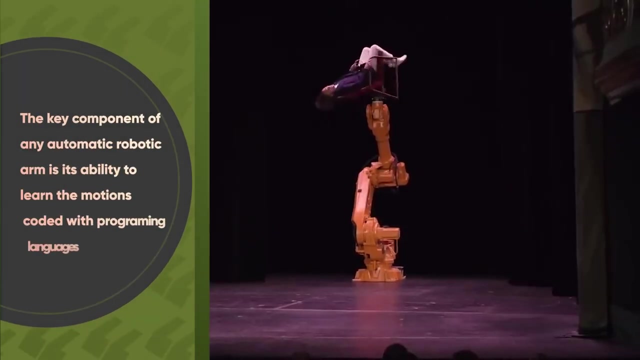 patrolling. So here is our RC robot tank, developed to run on rough terrains, with both night vision and thermal vision, wireless transmission, Programmable robotic arm using Arduino. Robotic arms have a wide range of application in industry automation and food automation industries. The key component of any automatic 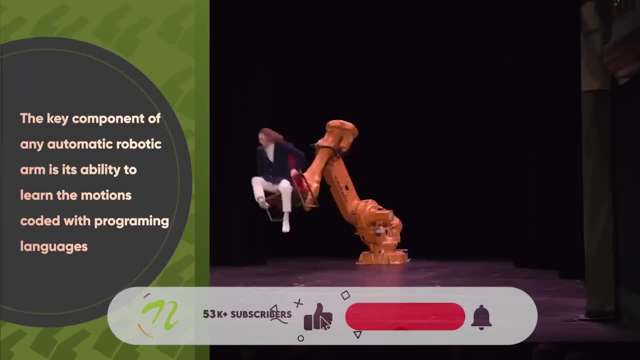 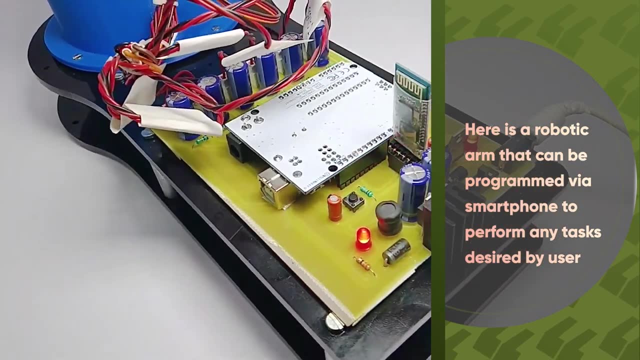 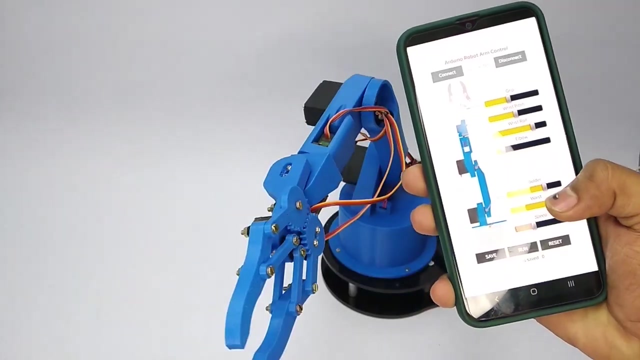 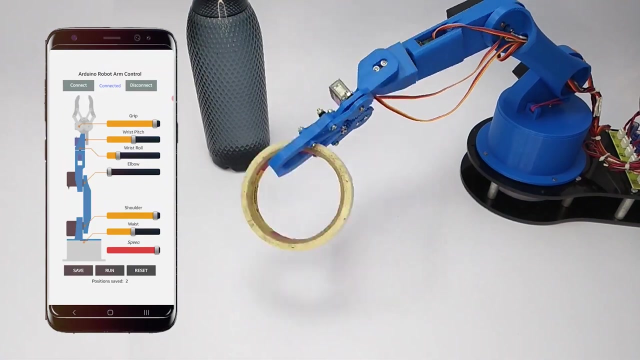 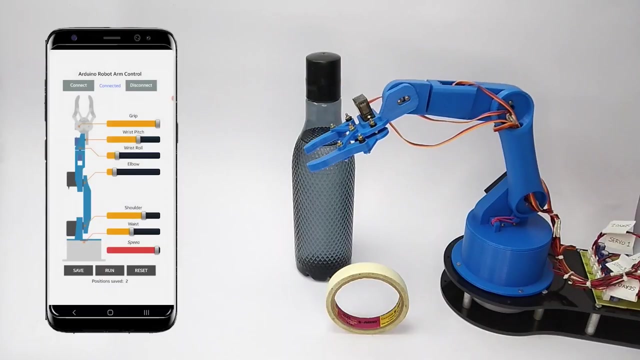 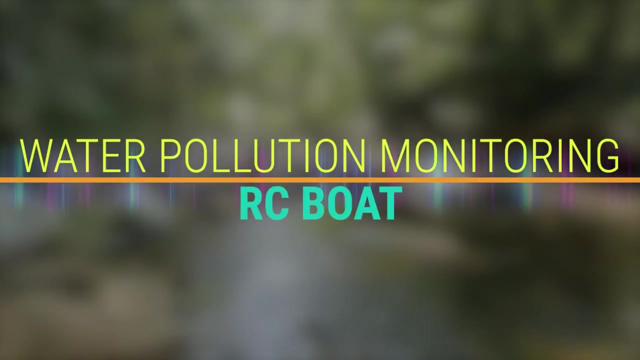 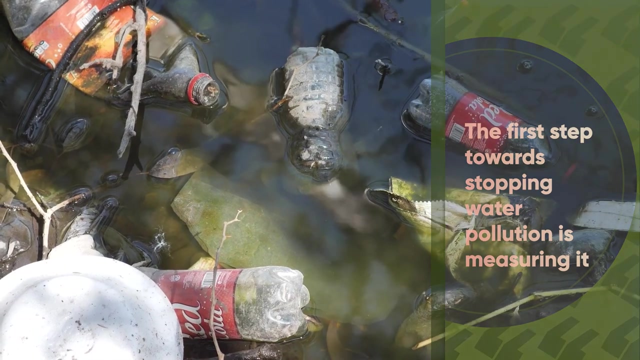 robotic arm is its ability to learn the motions coded with programming language. So here is a robotic arm that can be programmed via a smartphone to perform any task desired by the user. Water pollution monitoring RC boat. The first step towards stopping water pollution is measuring. 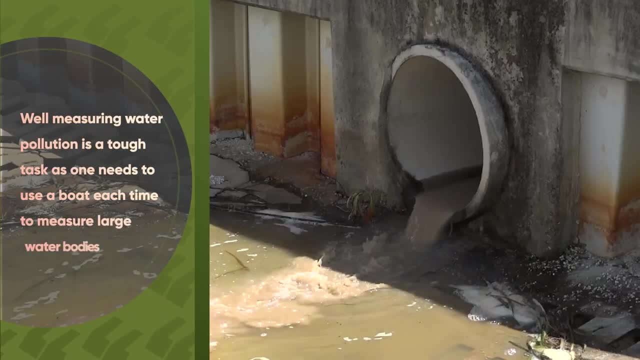 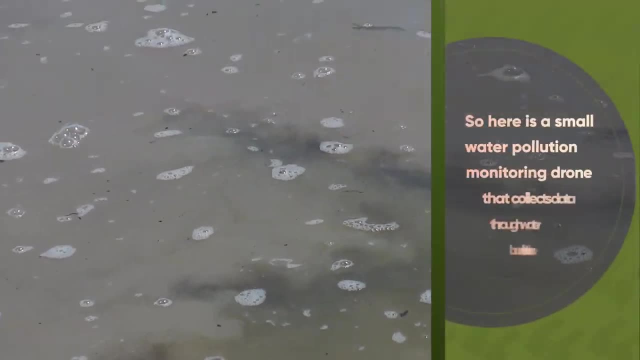 it Well, measuring water pollution is a tough task, as one needs to use a boat each time to measure large water bodies, So here is a small water pollution monitoring drone that collects data through water bodies with ease Water pollution monitoring RC boat. The first step towards stopping water pollution is measuring. 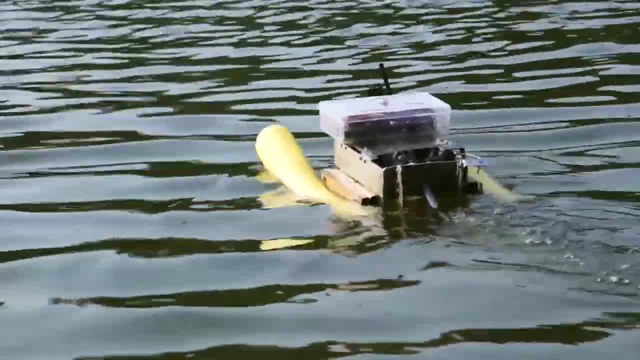 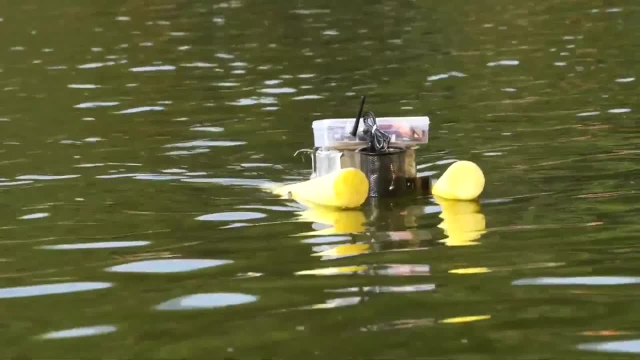 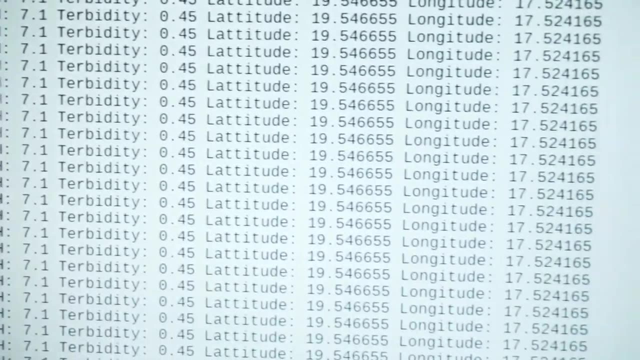 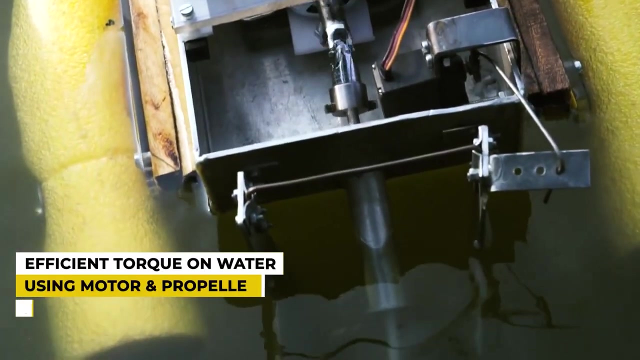 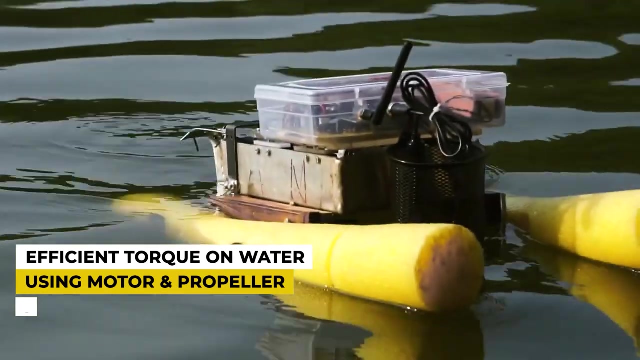 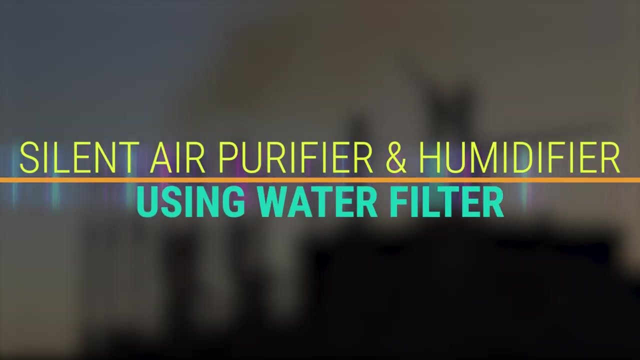 it. Water pollution monitoring RC boat. The second step towards stopping water pollution is measuring it. Water pollution monitoring RC boat. This is the way it is: Water pollution monitoring RC boat- The first step towards stopping water pollution. Silent Air Purifier and Humidifier using Water Filter. 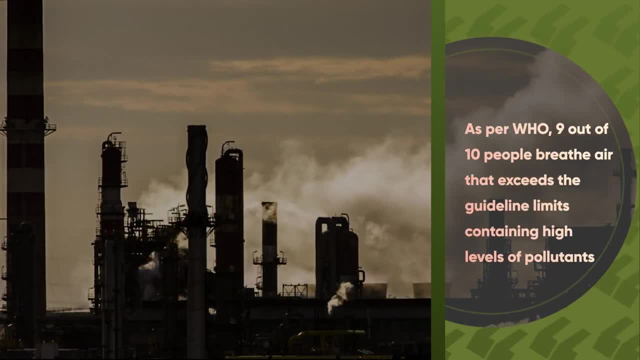 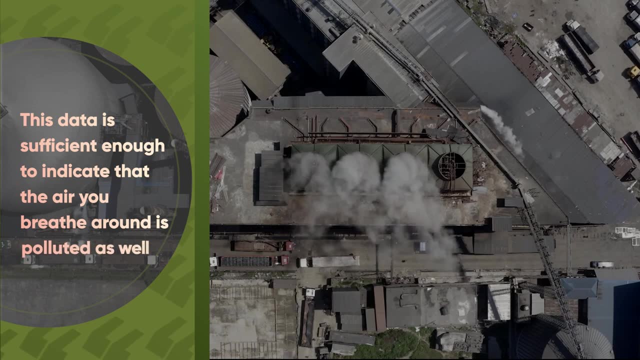 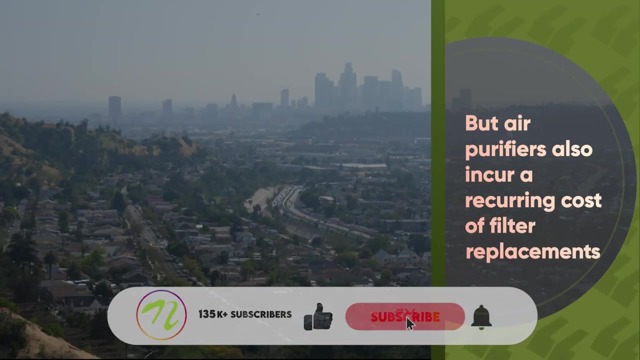 As per WHO, 9 out of 10 people breathe air that exceeds the guideline limits containing high level of pollutants. This data is sufficient enough to indicate that the air you breathe around is polluted as well, But air purifiers also incur a recurring cost of filter replacements. 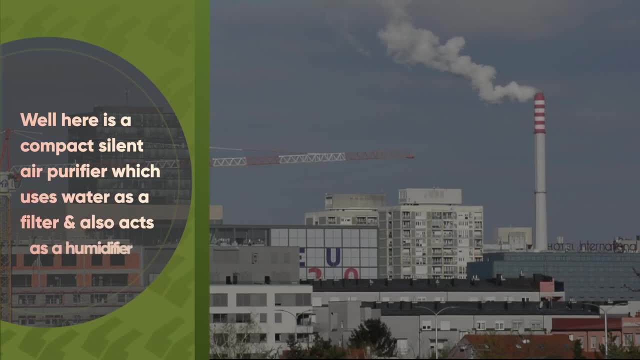 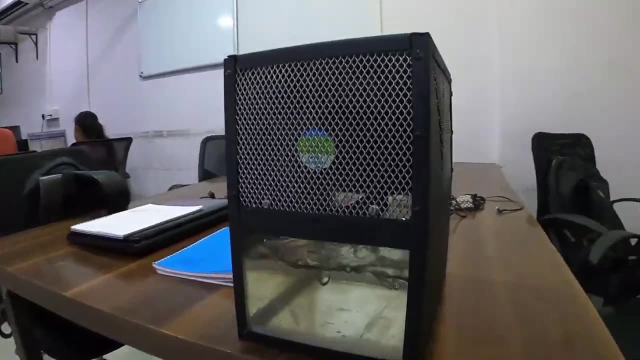 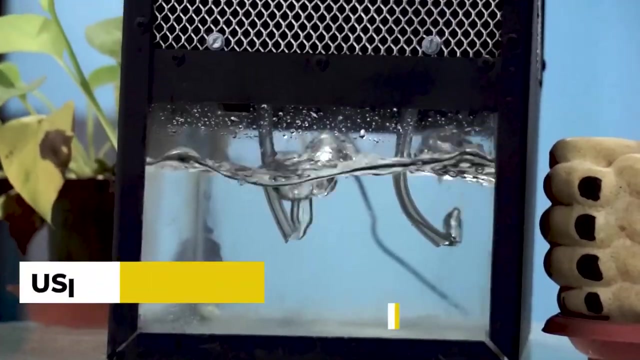 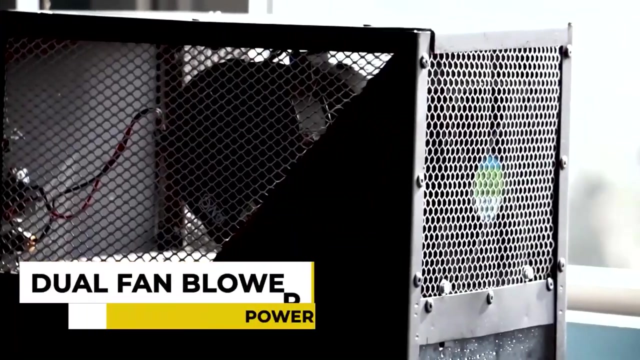 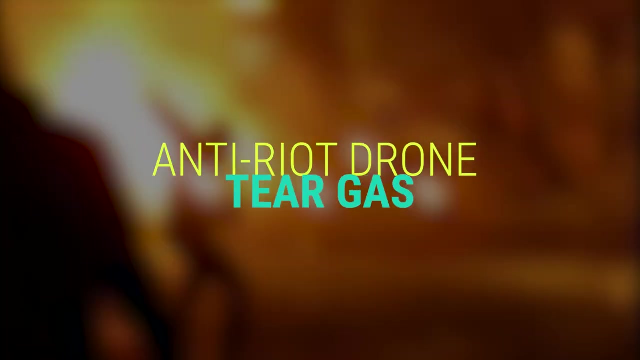 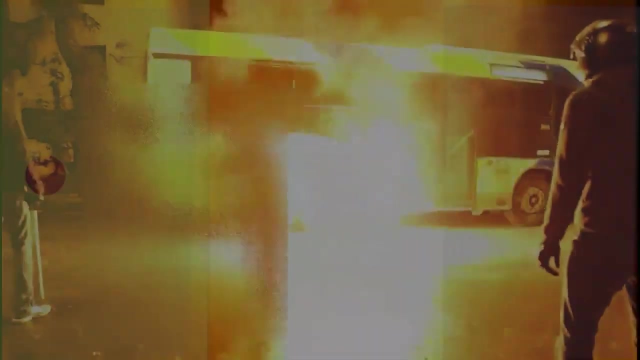 Well, here is a compact, silent air purifier which uses water as a filter and also acts as a humidifier. Anti-Ride Drone with Tear Gas. Ride control is a very tough and dangerous job. Security forces are at high risk of injuries while handling rides and protests. 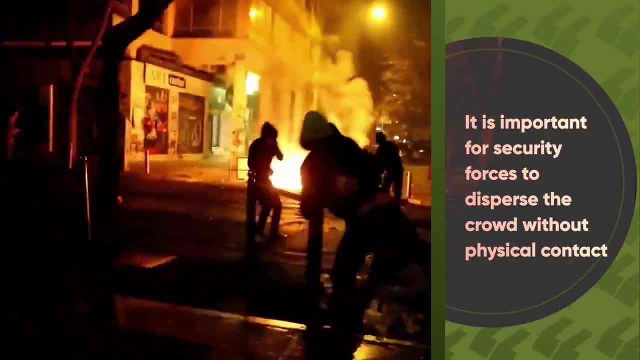 It is important for security forces to disperse the crowd without physical contact. So here is a high-tech anti-ride drone with tear gas which can be used to control the air. Anti-Ride Drone with Tear Gas. Anti-Ride Drone with Tear Gas. 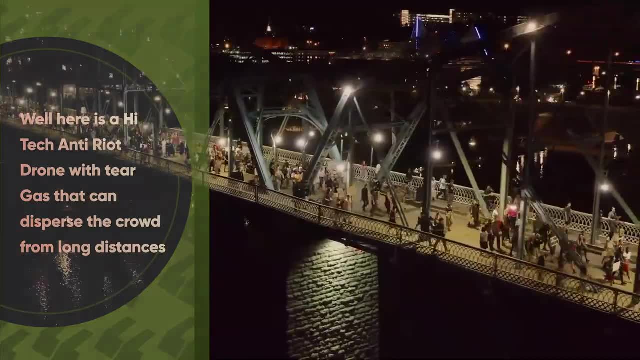 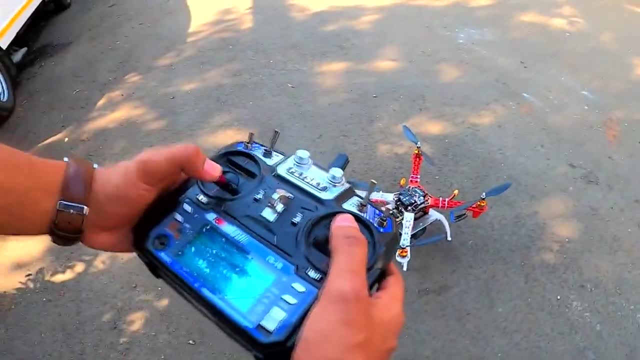 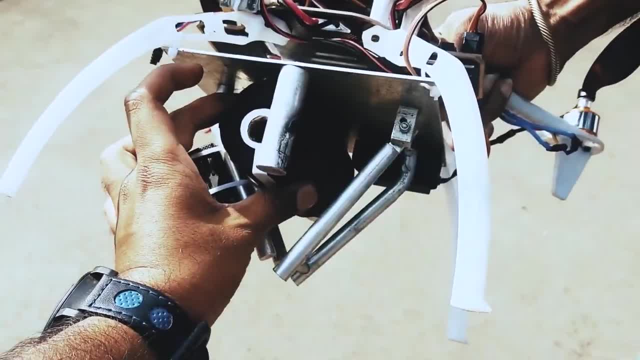 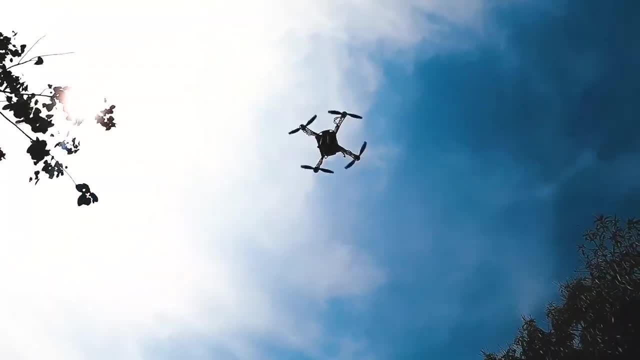 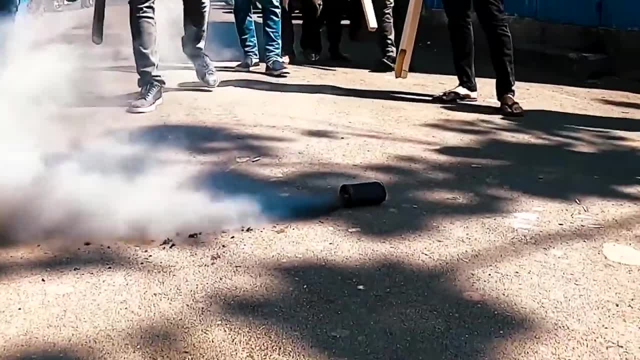 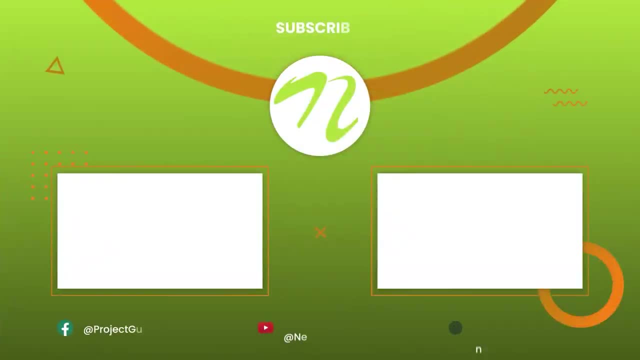 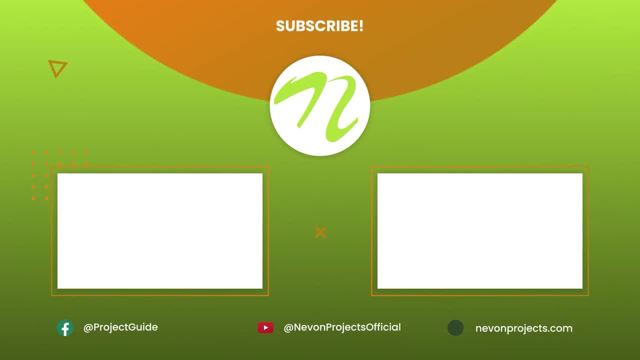 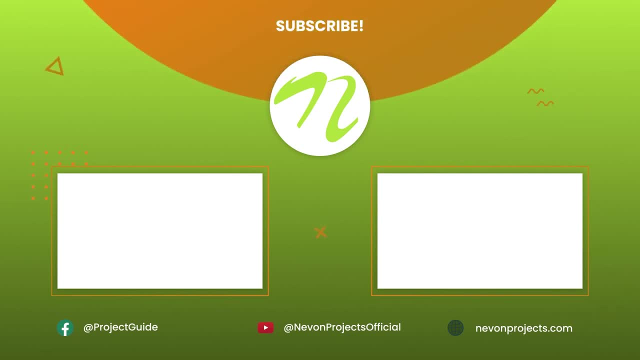